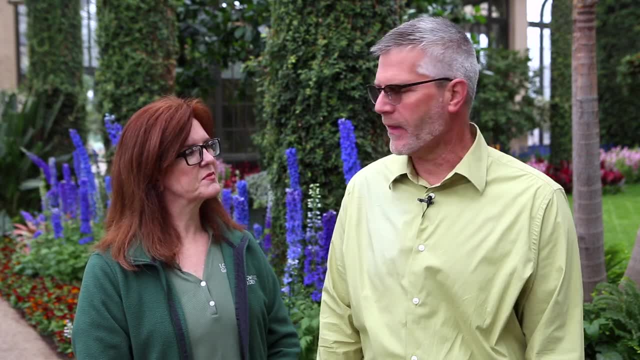 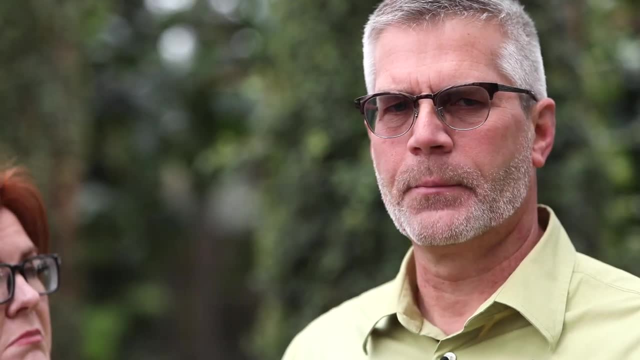 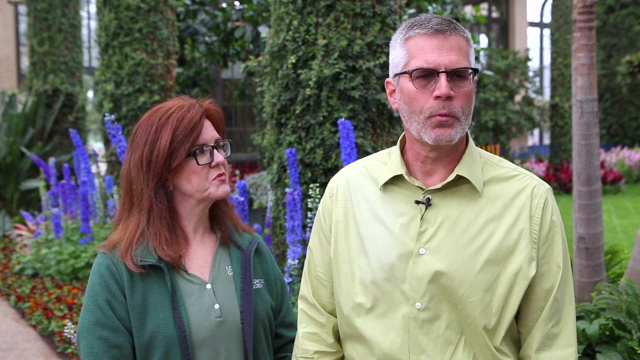 Gardens, there are over 5,000 species representing 11,200 taxa on display. How many plant species are there in the world? There are roughly 400,000 estimated plant species. We're constantly finding new and exciting species and developing hybrids through exploration and global breeding. 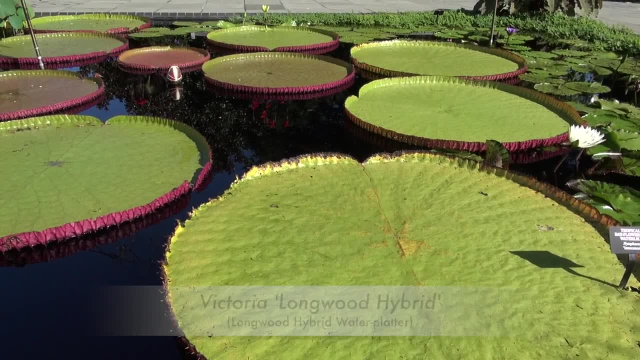 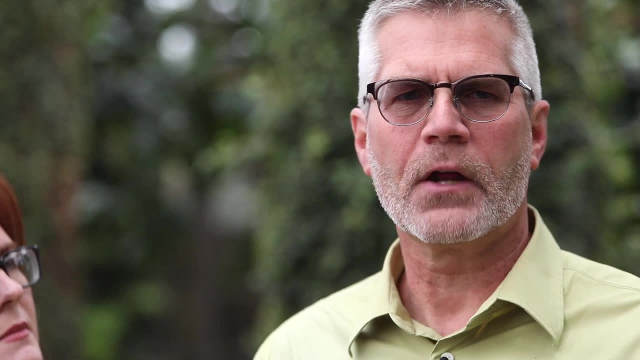 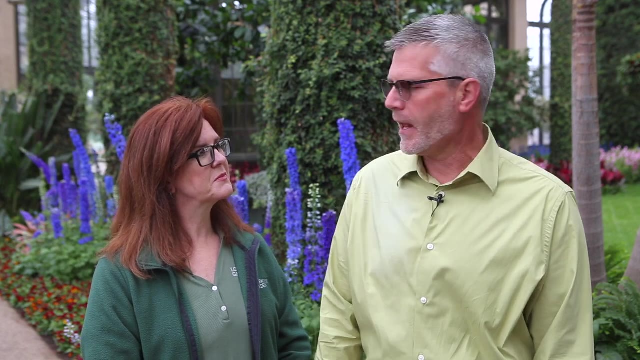 programs like the Victoria-Longwood hybrid. That is very intriguing. How did the plant world become this diverse? Many of the plants around us are vascular complex organisms, But to really understand the evolutionary path they took to become the towering plants we see today, let's start with their ancient ancestors and head over to the fern passage. 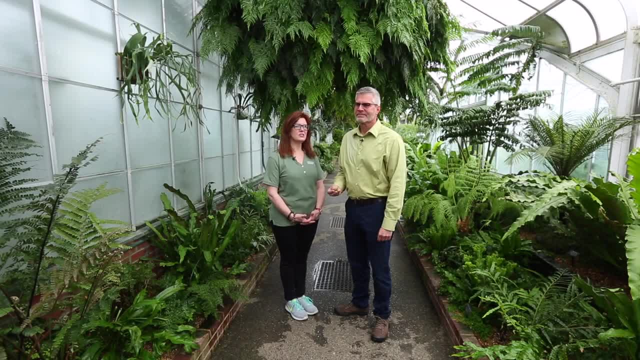 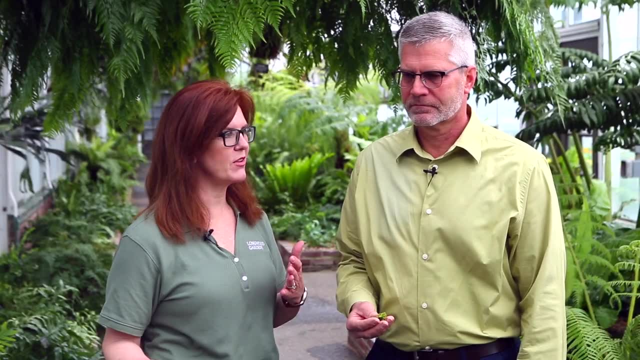 Great, Let's go. This is such a beautiful space, Jeff. I've always enjoyed the textures of the plants that are surrounding us here. What's interesting, though, is there are no flowers. Kelly, it's absolutely right. Many plants do not have colorful flowers- Ferns. 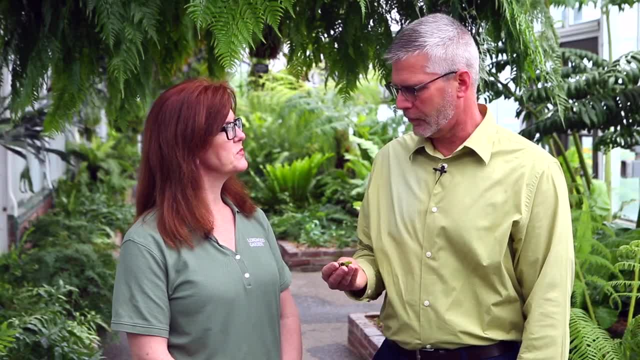 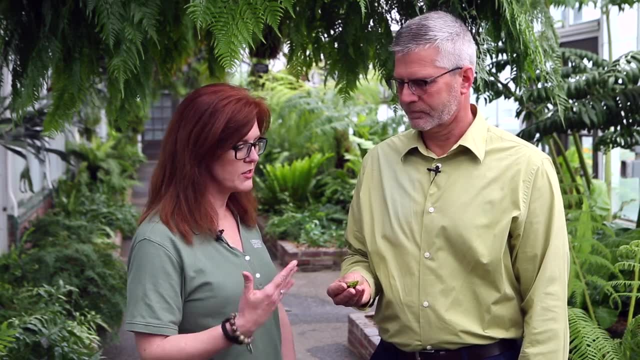 are actually a little more complex than the first group of organisms we're going to discuss, And we only have one variety of plants today. The Venus dwarf, which belongs to the Venus tree, of course has new white flowers. In fact, some plants have original flowers, If 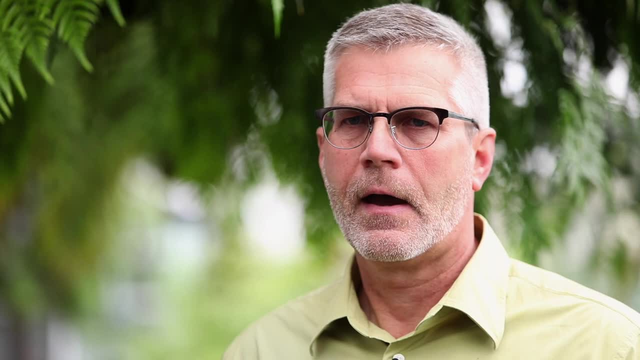 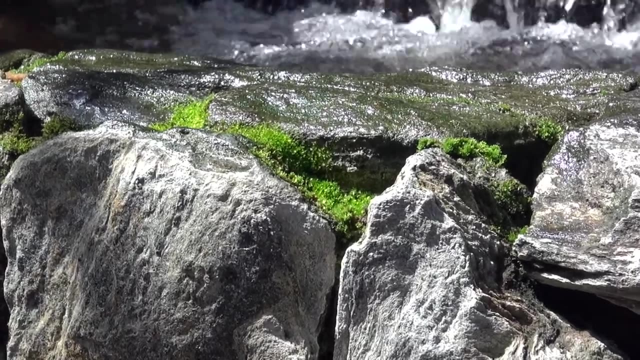 we take a closer look at the flower shape, you can see that the flower shape we're talking about here is not completely the same. It's the same, but with a different plante order, which is what we call the royal ummadi. The Indian overwhelmingly got their names till. 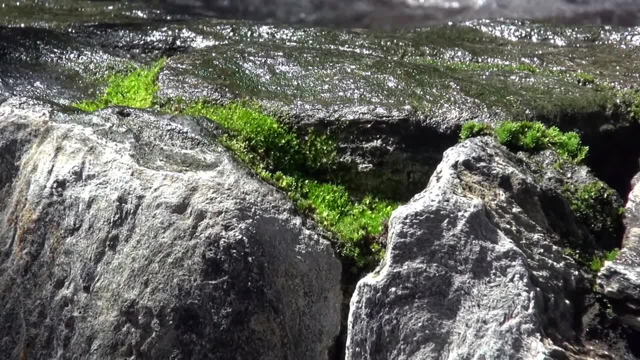 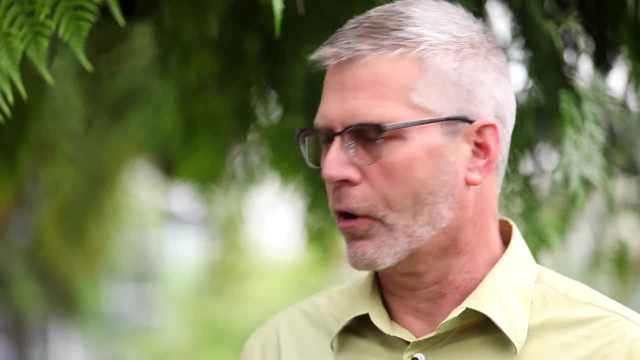 about 5,000 years ago, The Venus dwarf got four flowers, so they are still growing. yet the plants are growing And what we're seeing is more and more plant species are expanding on their cellular configuration. They are the ancestors of the plant kingdom. It 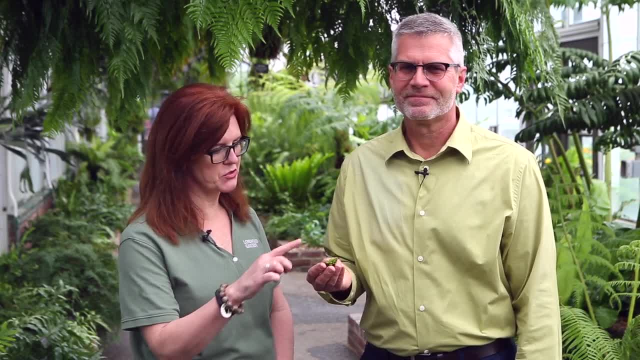 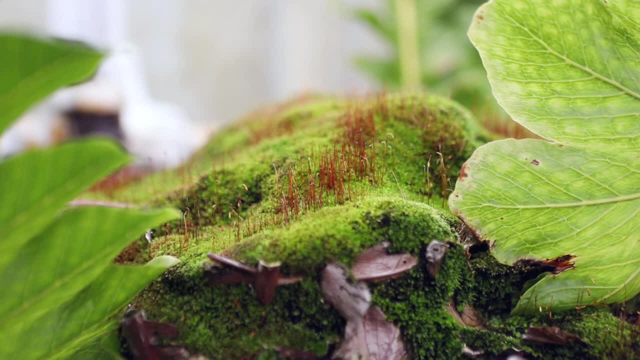 looks like something is about to bloom. What are these structures on the moss, Kelly? while they don't bloom, mosses use structures like these sporangia to reproduce, and many of them can be colorful and exciting to spot. That is very cool. The next plants to develop were many of the larger seedless. 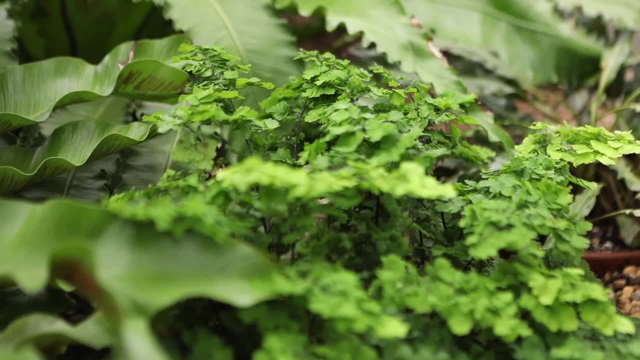 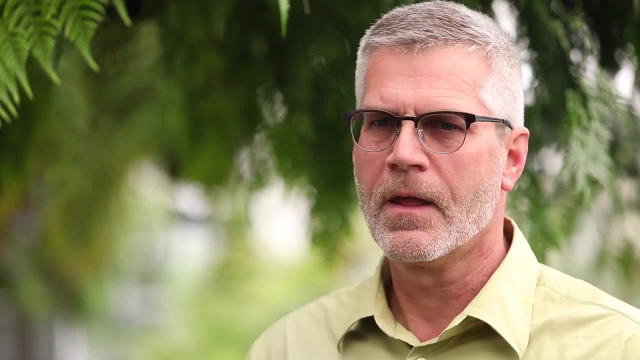 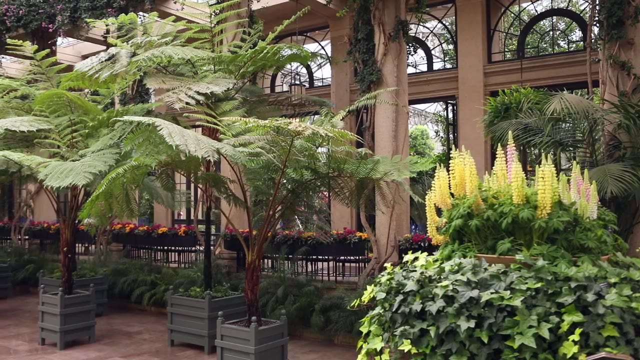 vascular plants like the intriguing lycopod and many of the pterophytes or ferns and fern allies. These early vascular plants first evolved nearly 400 million years ago. Some of my favorite plants in this category are the bird's nest fern Asplenium astrolasticum and, of course, the tree fern Dixonia. 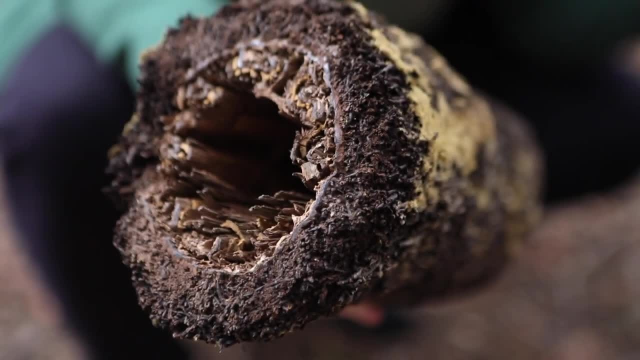 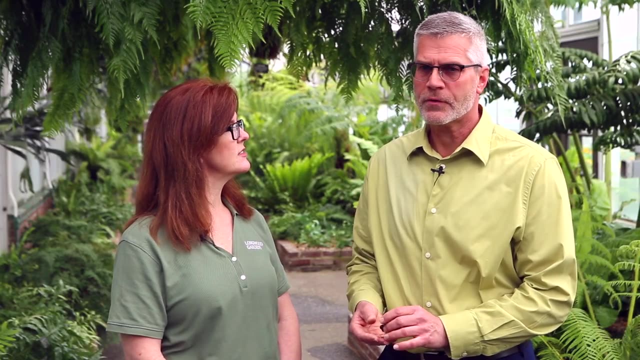 They are not only beautiful plants, but have some amazing bark patterns which are used in artwork and as a growing media for orchids. And what plants then came after the mosses and ferns? Let's venture outside to experience the world of flowering plants. Let's go. 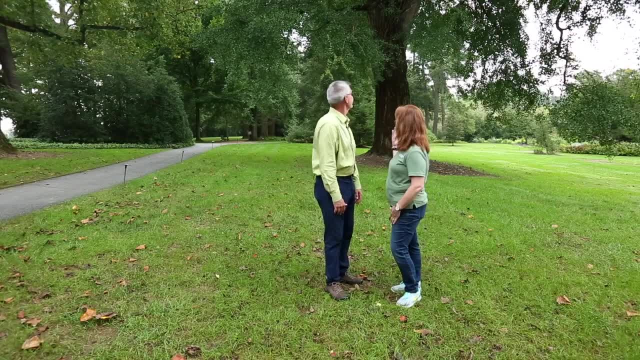 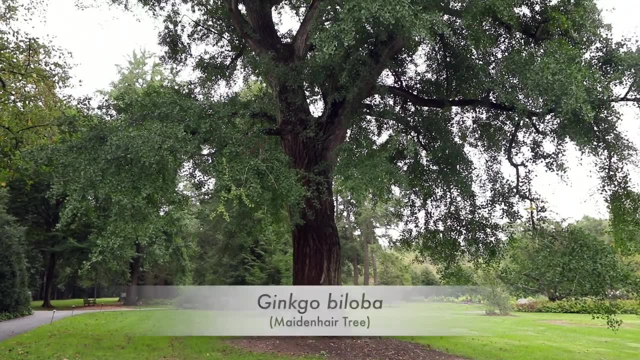 We are in Pierce's Woods at the base of one of my favorite trees on the property. Can you tell me about this tree Sure? This is the Ginkgo biloba or maidenhair tree. It's a gymnosperm and gymnosperms are woody plants. What makes it a woody? 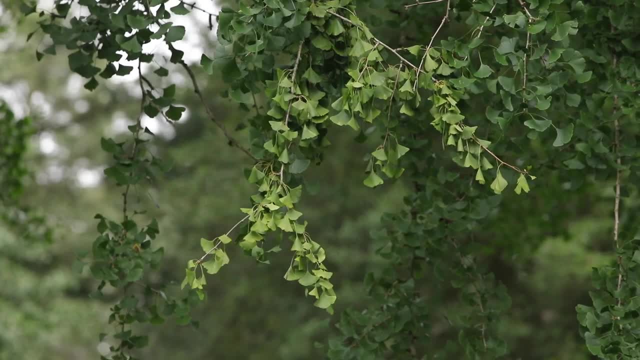 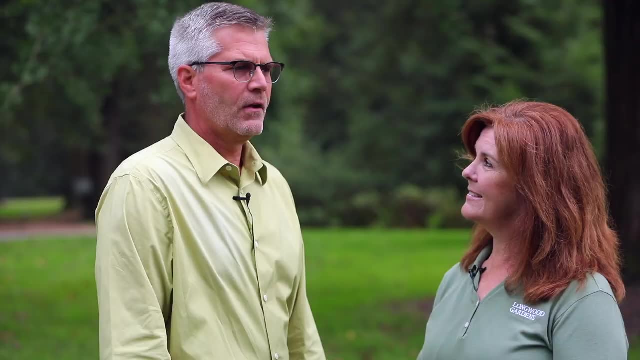 plant, Jeff, It's a woody plant. because of secondary growth, It has additional layers of xylem and phloem, the vascular system, as well as a presence of lignin. What is lignin? So lignin is a chemical compound that is deposited on plant cell walls. 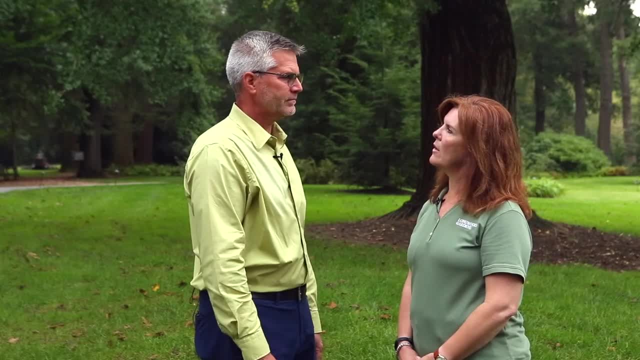 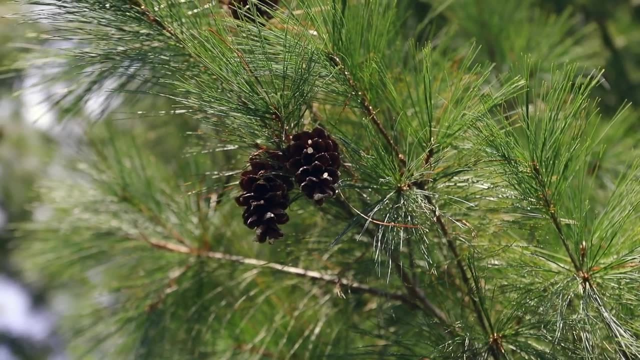 and it makes the cells rigid. So what are other features of gymnosperms? Gymnosperms have naked seeds, The seeds are in cones and they're typically wind pollinated plants. Alright, Can you give us some other examples, Jeff, of gymnosperms? Sure Things like conifers, pine, spruce, fir, juniper and sequoias, as well as cycads and ginkgos. Well, I know that cycads and sequoias are quite old. How old is the Ginkgo family? 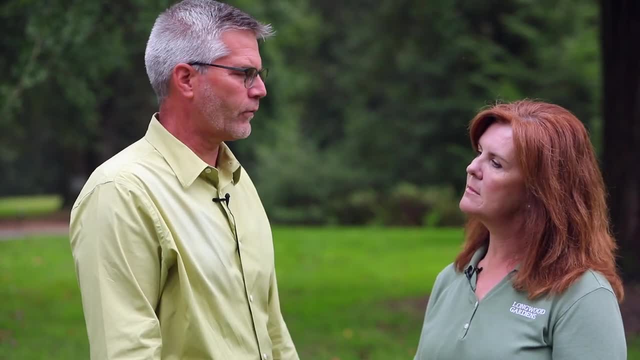 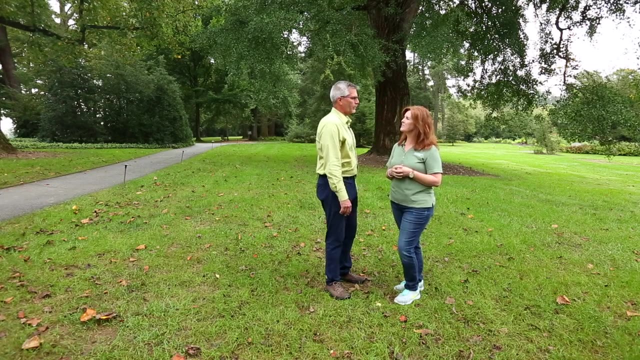 Fossil records tell us that the Ginkgo family is about 245 million years old. What about this Ginkgo? Any idea how old this tree is? Well, our best estimate is that it was planted in the 1800s. Oh, how about that? Gymnosperms are the cone-bearing plants. 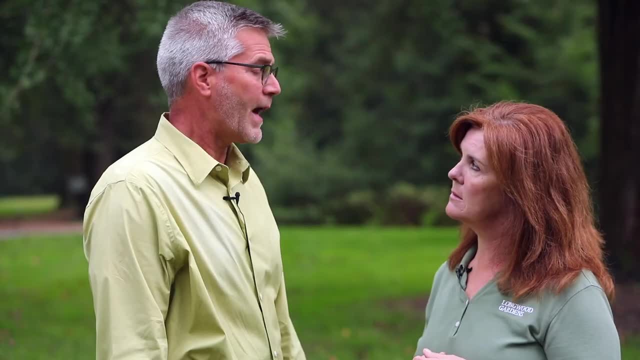 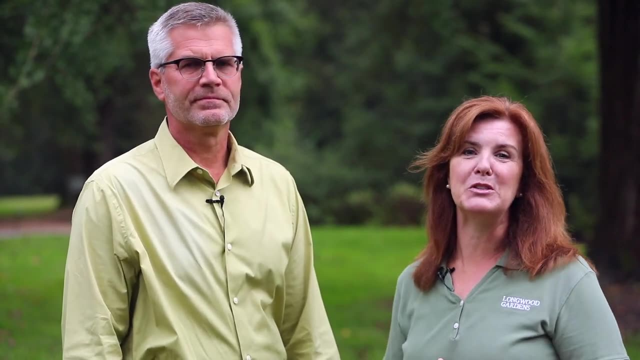 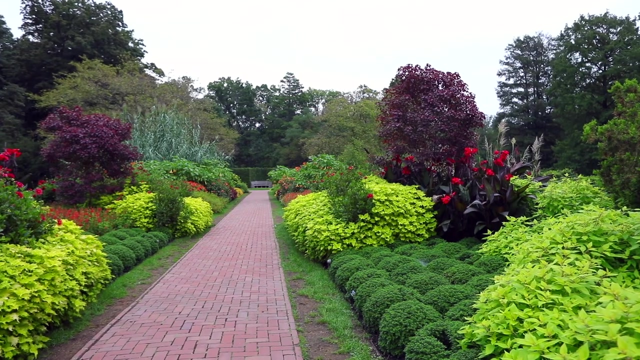 as you have explained. but what about the flowering plants? The flowering plants are angiosperms. Let's look at those. next Great, Let's travel to a beautifully flowered area here at Longwood Gardens: the Flower Garden Walk. Here we are at the Flower Garden Walk, surrounded by these incredible blooms, Most of the plants. 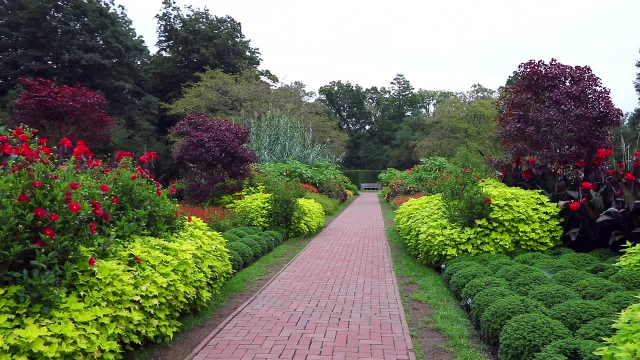 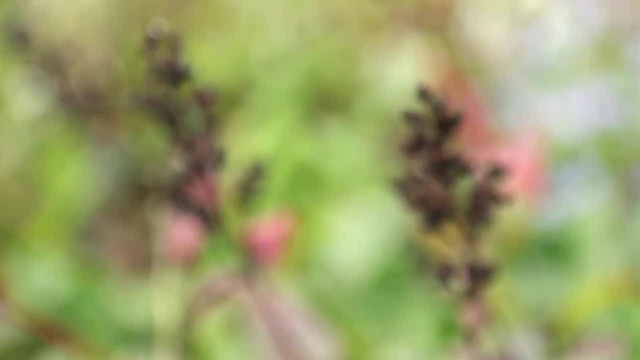 that you see in flower are angiosperms. What are angiosperms? Angiosperms are the flowering plants, those with a true flower that will form seeds enclosed in a fruit. These are the last plants to evolve. How many angiosperms are there? They're the largest group in the 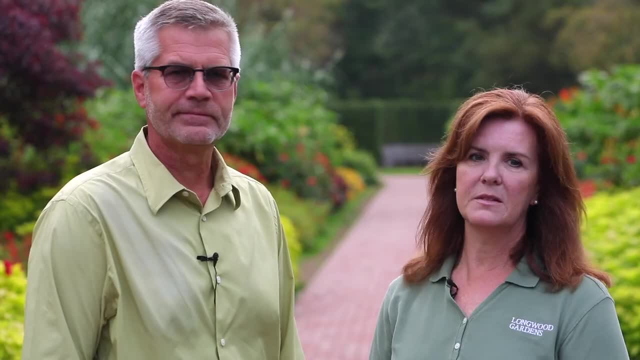 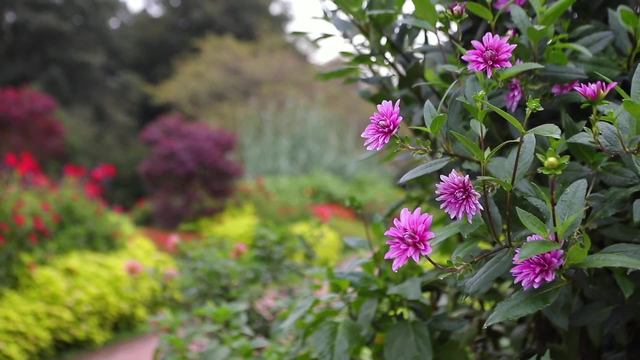 plant kingdom, with about 250,000 species. Other than these plants that we see right here, what other plants are angiosperms? Most of the plants that we use in gardening and landscaping are, as well as plants in fruit and vegetable production and plants.